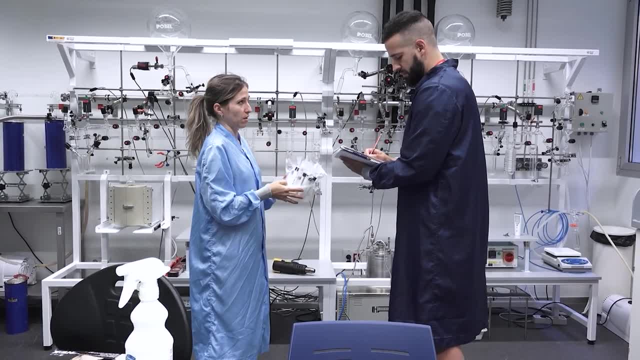 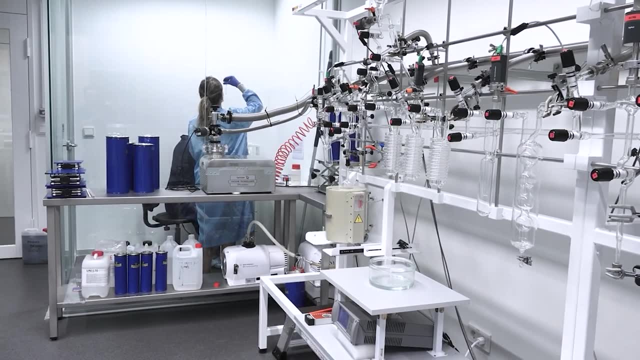 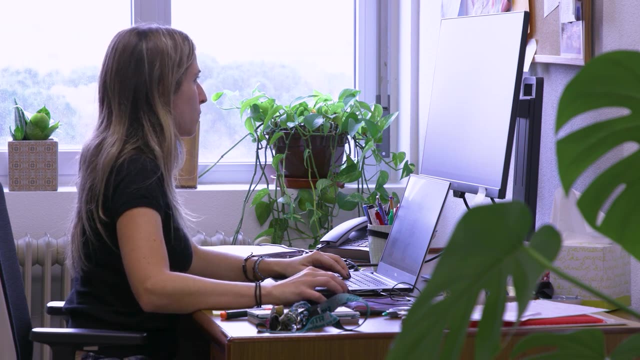 we can access two elements that are important for climate reconstruction: Oxygen isotopes and radiocarbon. While the first holds information about changes in the climate, the second tells us when the organism lived Like. so Each layer in the sediment where foraminifera are. 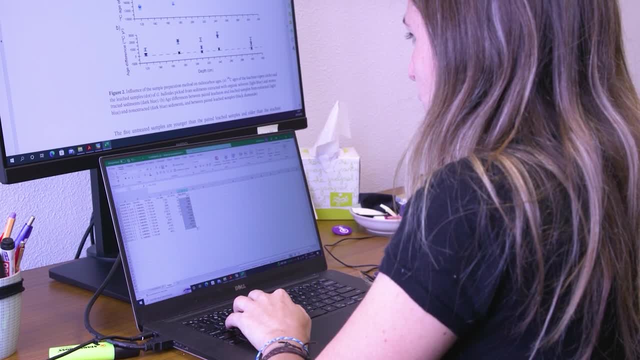 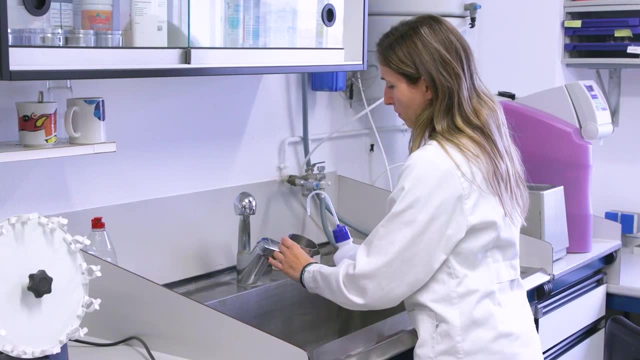 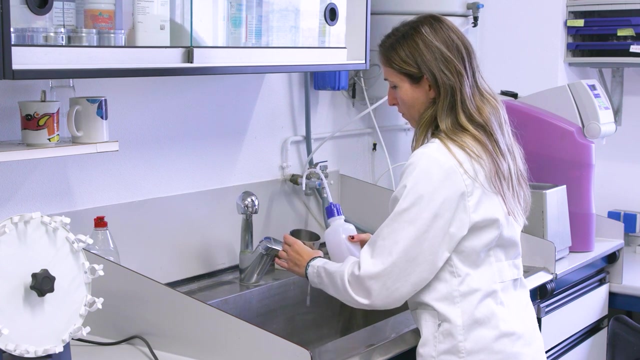 present can be assigned an age. Moreover, fossil foraminifera shells are extremely useful in paleoclimate research in several other ways. For example, their abundance is used to get an idea of the productivity of the water at a certain period, Or the species distribution in the fossil assemblage is very useful to 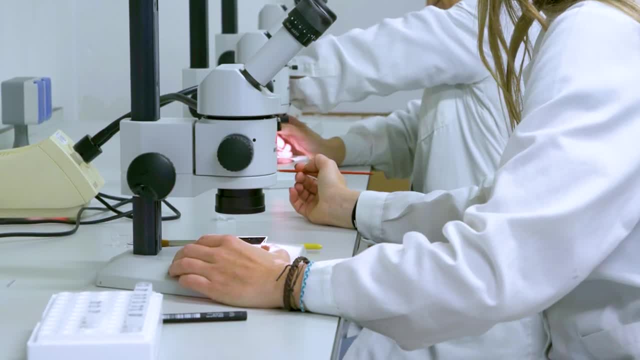 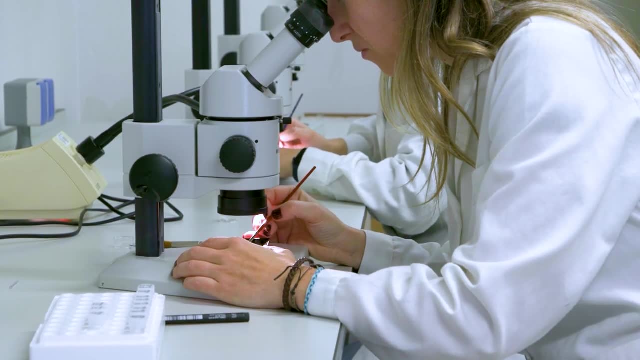 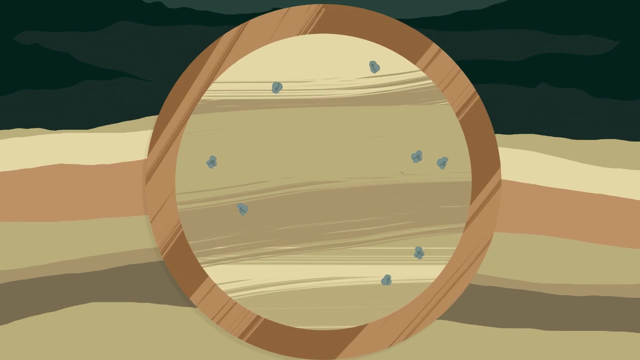 get information on the characteristics of the water mass in which they live. And finally, the geochemical composition of the foraminifera shells can give us specific information and key variables for climate changes, like temperature or sea ice volume. It gets more complicated. There are also other organisms living in the sediment. They can 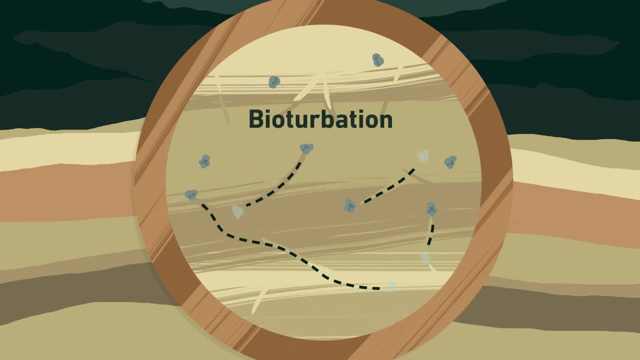 make a mess in the deposited material, a process called bioturbation. This is when the shells of the foraminifera come in handy. While some stay in place, others get moved around. To get an idea of the degree of disorder, it is useful to look at the radiocarbon concentration. 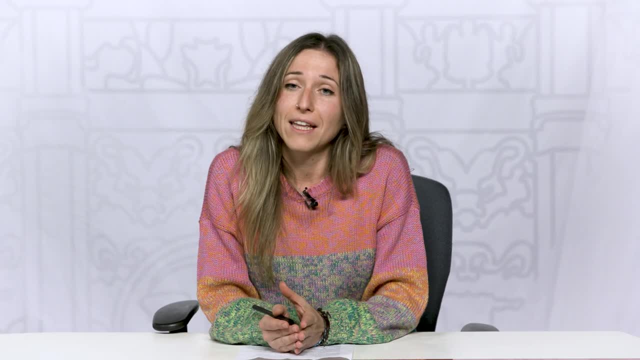 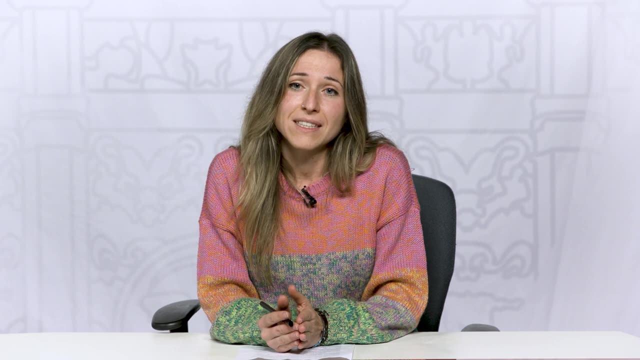 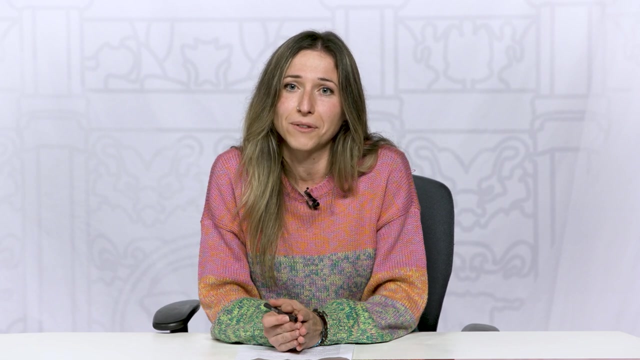 in the different foraminifera species. And finally, it gives us information on the radiocarbon signature of the water mass in which the organism lives. Sometimes it happens that different species that live in the very same water mass keep very different radiocarbon signatures. When this happens, new questions? 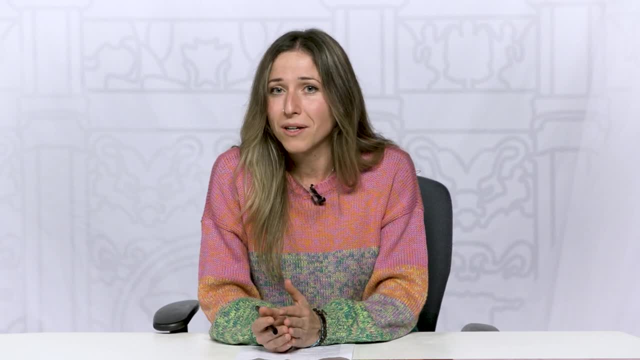 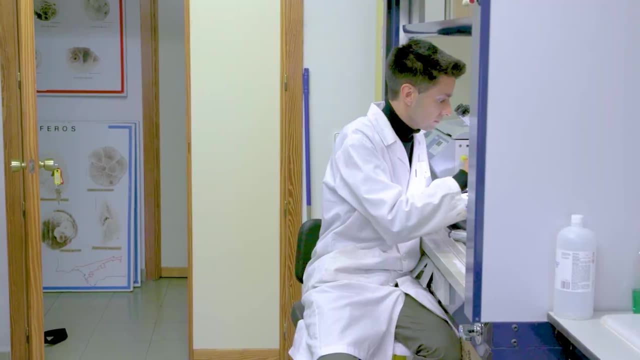 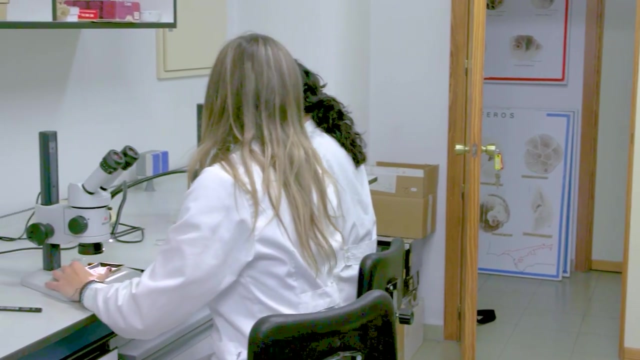 arise. For example, did something happen to one of the species, And did this happen before they made it to the seafloor or afterwards? This is exactly what this case study focuses on: Bioturbation and how this process impacts the chronostratigraphic control we have on. paleoclimate reconstructions.